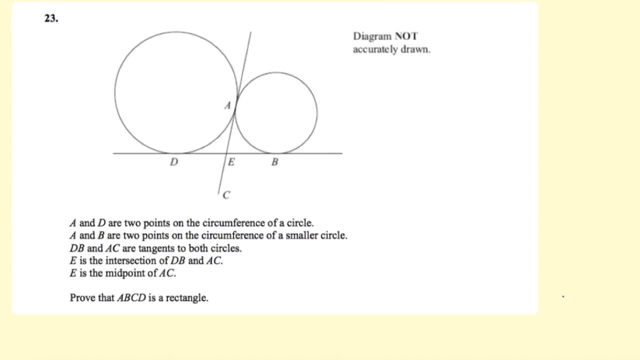 Hey, what's up guys? In this video I'm just going through this exam problem. That's all I'll be going through. This is an exam problem from one of the practice sets, So let's get straight into it. The question says: A and D are two points on the circumference of a circle. A and B are two points. 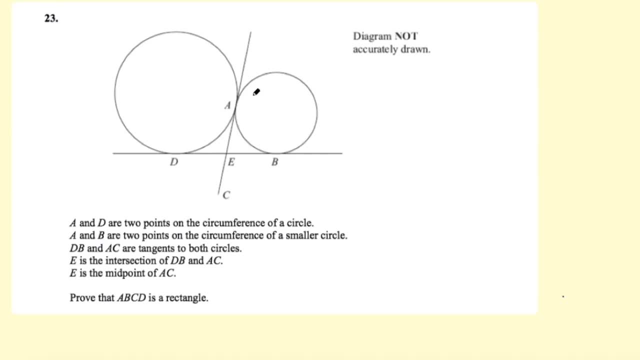 on the circumference of a smaller circle. So here we have the larger one and the smaller one. D, B and A C are tangents to both circles. So here's A C and this is D? B, and they're both. 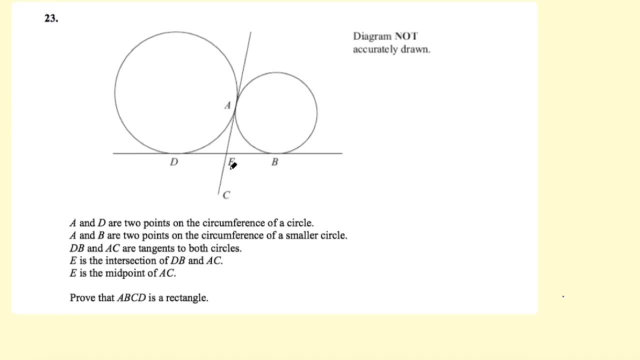 tangents: E is the intersection of D, B and A C. E is the midpoint of A, C. So here's E, and we're told that it's the midpoint. So A, E and E, C must be equal. and it says: prove that A, B, C, D is a. 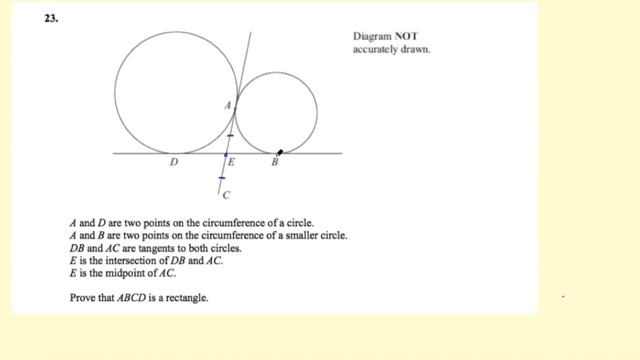 rectangle. Okay, so here's A, B, C and D, and we need to prove that is a rectangle, So let's draw that in. Okay, there we go. Alright, so let's think about a rectangle. What makes a rectangle? What are the? 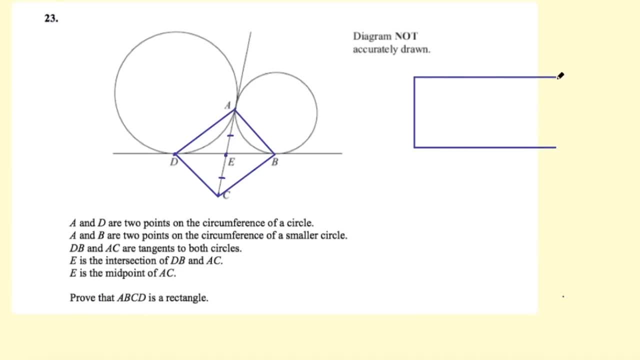 conditions of something being a rectangle. Well, a rectangle needs four 90 degree angles. Okay. also, its diagonals are equal in length. So if you take a rectangle and measure the diagonals, they're always going to be equal and they meet at the 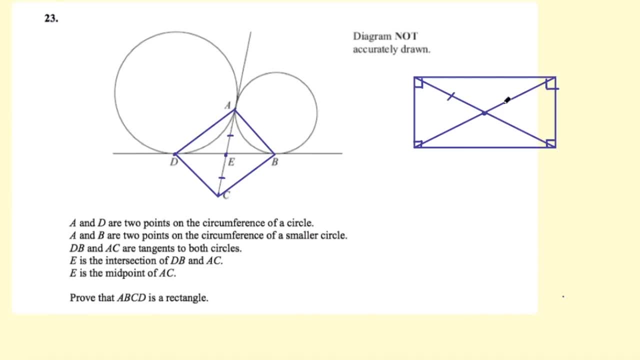 midpoint of the rectangle and also these lengths are equal. So the rectangle, the diagonals, meet at their midpoints and they are bisected. So each length here is equal. So we can either prove that this rectangle has four 90 degree angles or that the diagonals 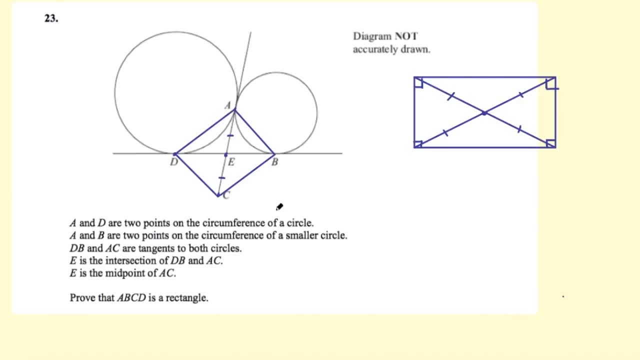 are equal in length, and if we can do that, we can prove that A, B, C, D is a rectangle. Alright, so let's have a closer look at this diagram. now We're told that A, C and D- B are tangents. Now there's a rule about tangents meeting at a point, an external point to a circle, and that says that they are equal in length. 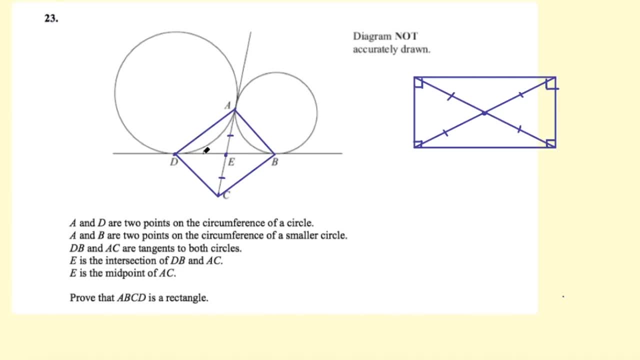 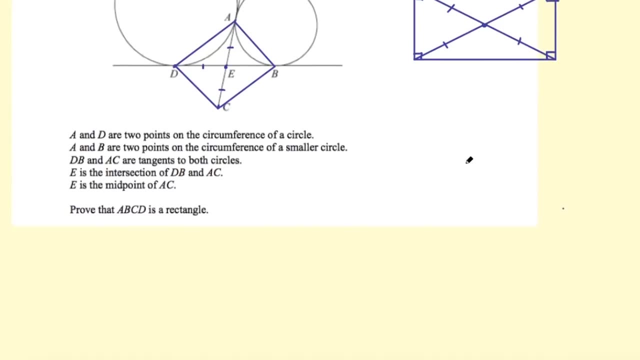 from where they meet the circle to that intersection point. So in other words, D E is equal to A? E. Let's let me explain that a bit more. So it's pretty easy to prove. So if you have a circle and you have two tangents to that circle, let's just say they're like this and they: 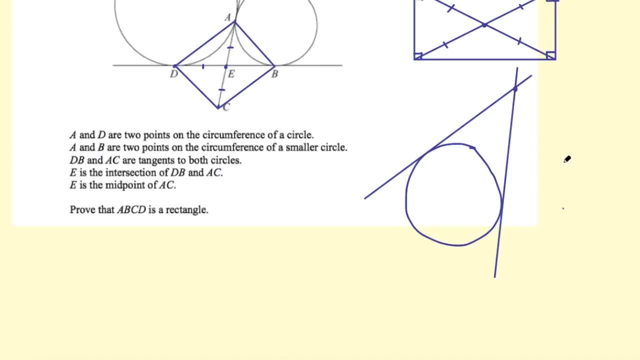 meet at some point outside of the circle. we can pretty easily prove that they must be the same length in here where they from the point where they meet the circle to the intersection point. If we take the center of the circle here and we draw the radii. 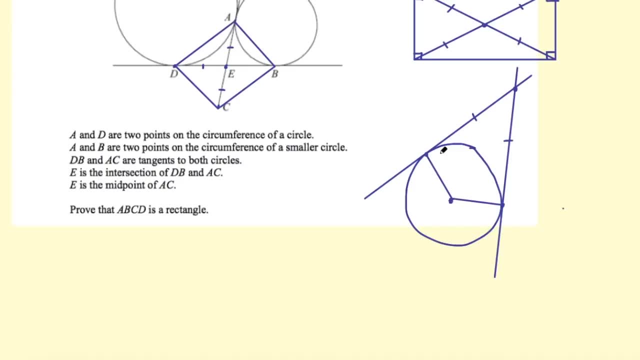 to the tangents. Now a radius meets the tangent at 90 degrees always, and because it meets at 90 degrees we can draw a straight line in here from the intersection point to the center of the circle and we can use the idea of congruent triangles because the radii are equal in length. 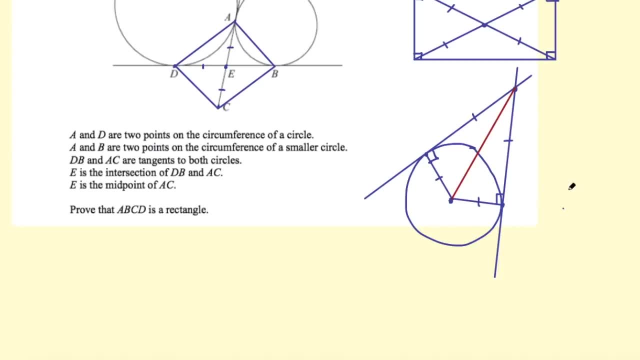 obviously because they're both a radius of the same circle. This line in here is the same length because it belongs to both triangles and there's a rule about right angle triangles that if the, the hypotenuse and one leg are the same length, then both triangles must be congruent. So because 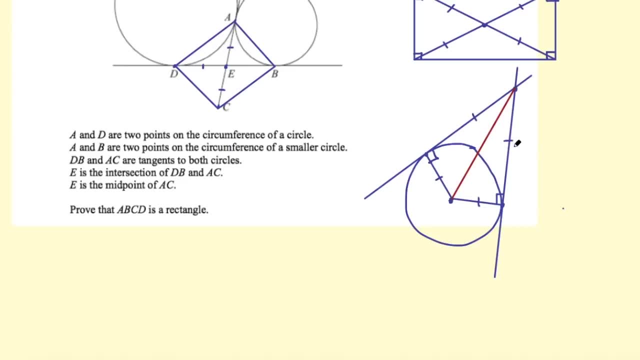 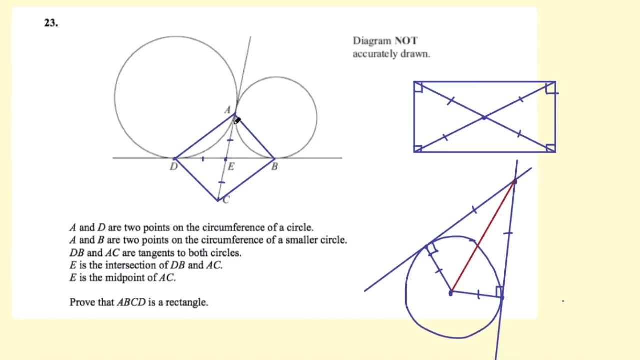 these two triangles are congruent. they're not congruent, So we can use the idea of congruent triangles. These lines in here are the same length. So we know, based on that rule, that DE and AE are the same length. and also we can use that same rule to say that EB equals AE and AE also equals EC, because 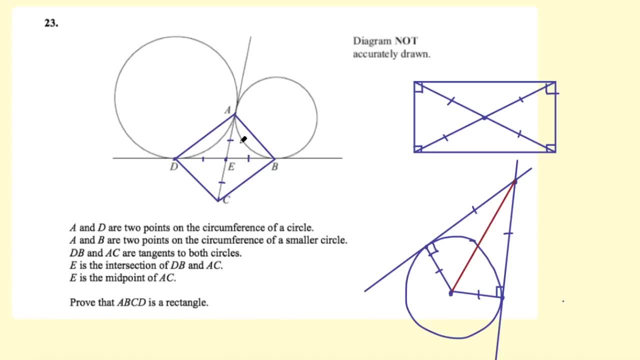 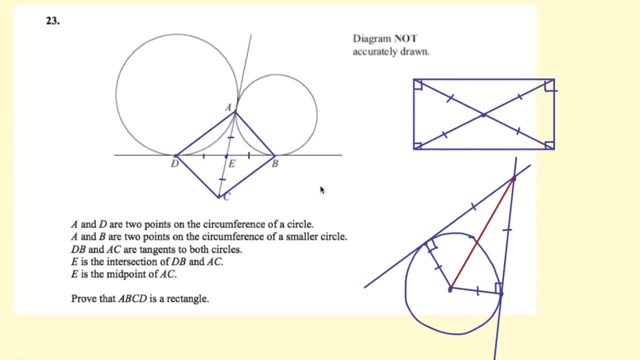 we're told that E is the midpoint of AC, So all of these lengths are equal. that means AC equals DB and as a result of that we can draw a straight line in here from the intersection point to the center of the circle. So, as I said before, if the diagonals are equal and they bisect each other, 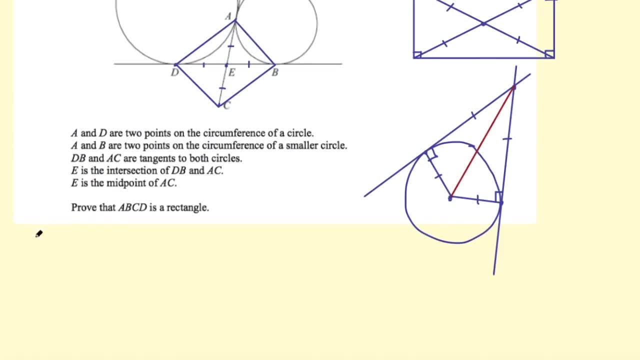 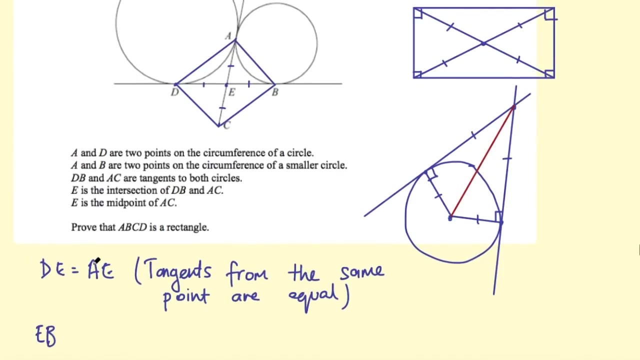 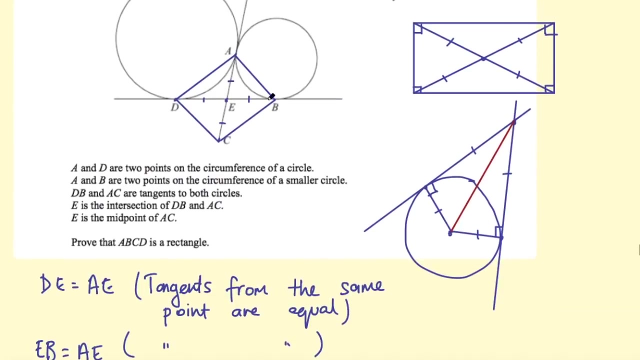 then it must be a rectangle. So let's go ahead and write some of this down and prove that it's a rectangle. So what we've said is that DE equals AE and we can say that tangents from the same point are equal, and also EB equals AE for the same reason, because AB and DB are also tangents to the. 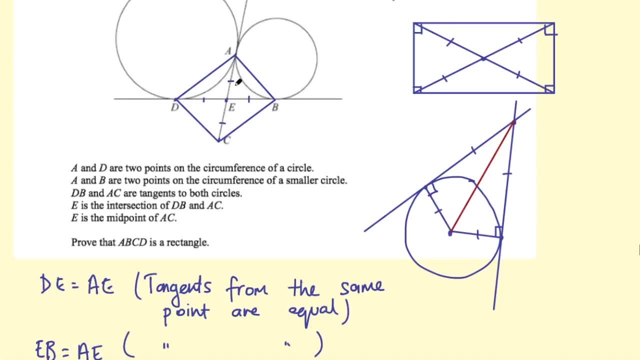 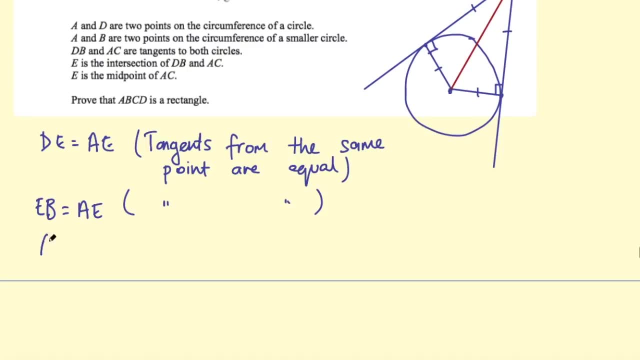 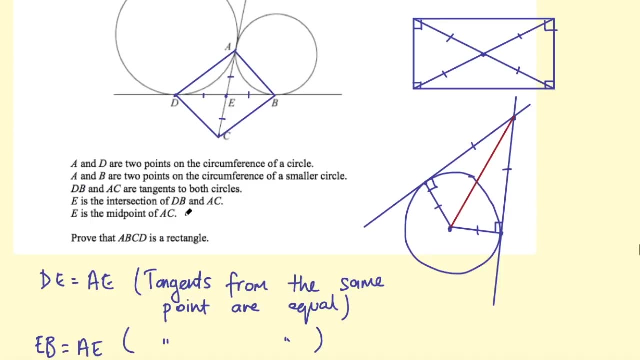 smaller circle. So these two lengths in here are equal. So we can say that DE equals AE and we can say that DE equals AE, and also we're told that AE equals EC. So this length equals this length and we're given that in the question because we're told that E is the midpoint. So we can just say that's given. 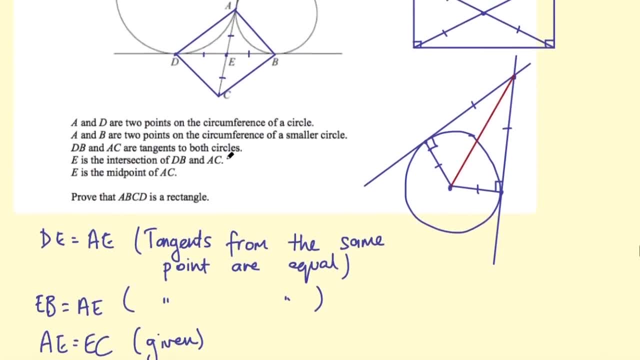 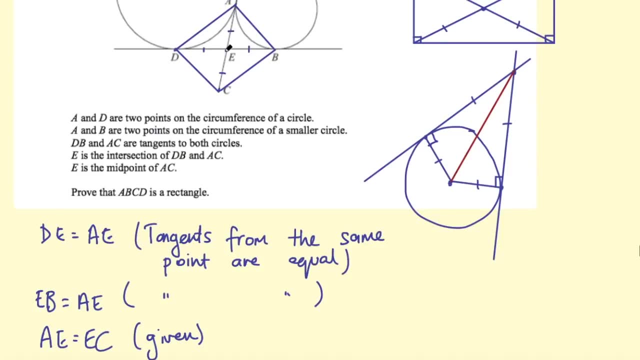 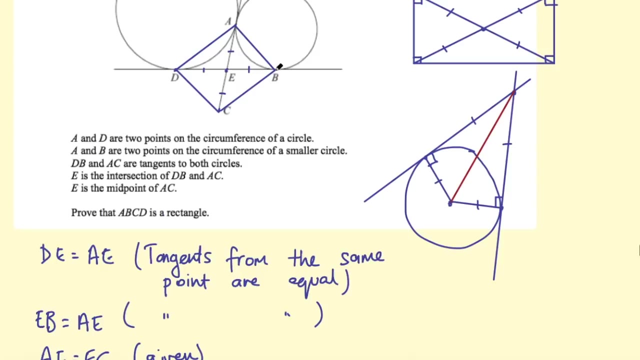 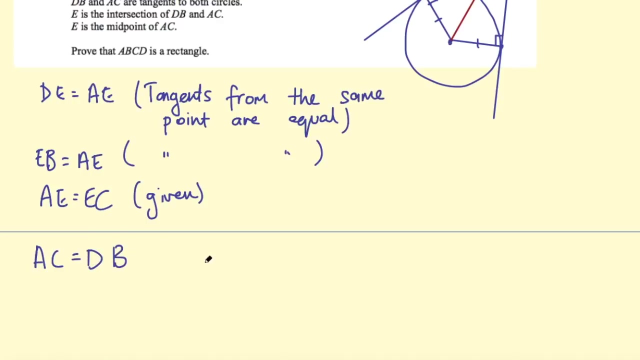 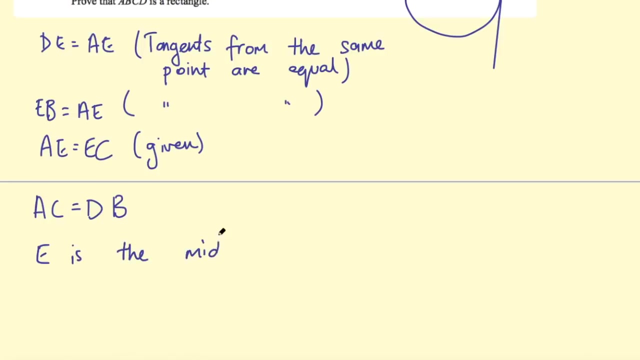 and so if DE and EB both equal AE, then DE also equals EB, and if all of these lengths are equal, then AC must be the same length as DB, So we can say that AC equals DB. Also, we can say that E is the midpoint of both AC and DB. 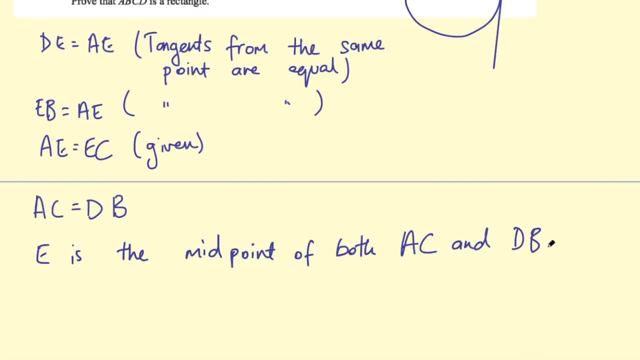 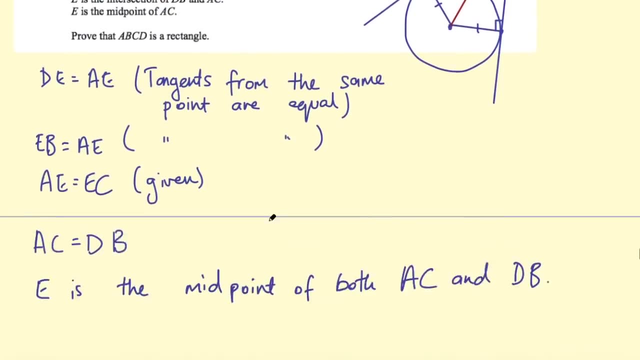 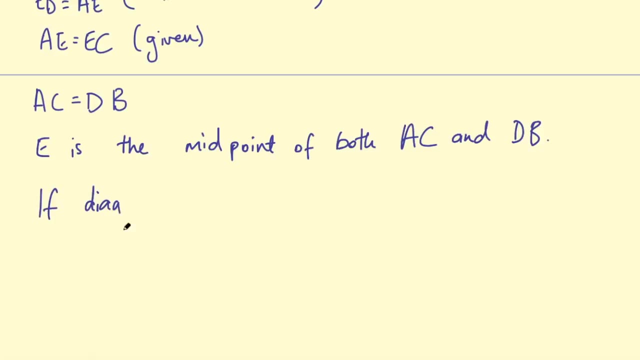 and DB, because if these two lengths, DE and EB, are equal, then E must be the midpoint of DB, And so we can also say that if diagonals of a quadrilateral are equal. and so we can also say that if diagonals of a quadrilateral are equal and.